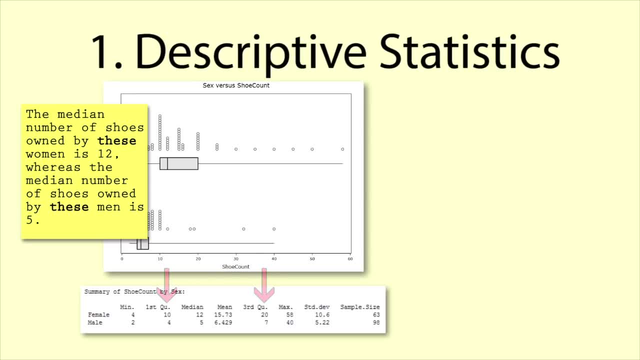 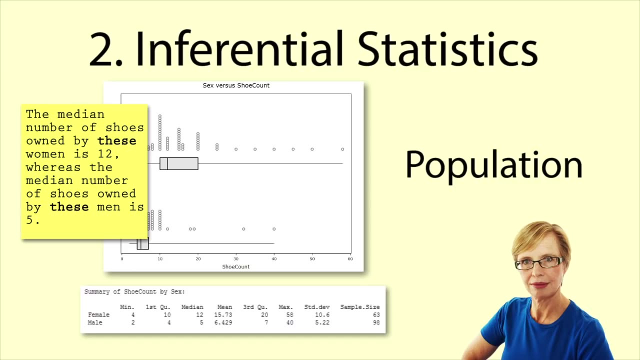 such as the mean and interquartile range. Descriptive statistics can help us identify relationships and patterns. Descriptive statistics do not draw conclusions beyond the data we already have. Inferential statistical analysis does allow us to make conclusions beyond the data we have. 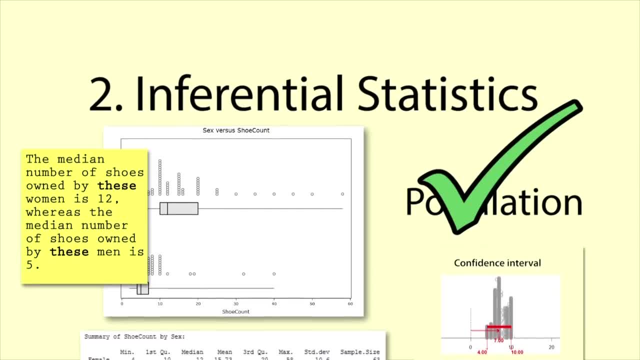 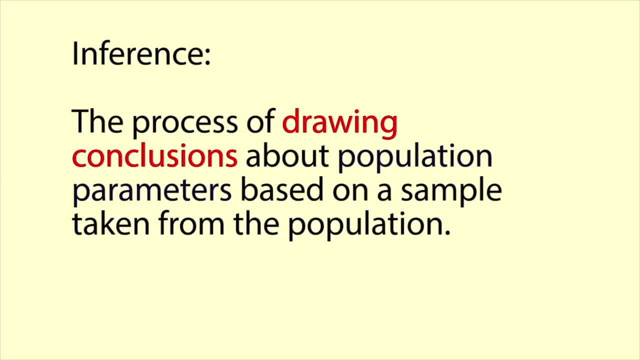 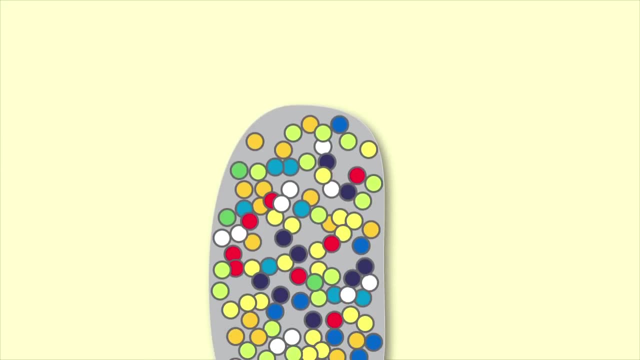 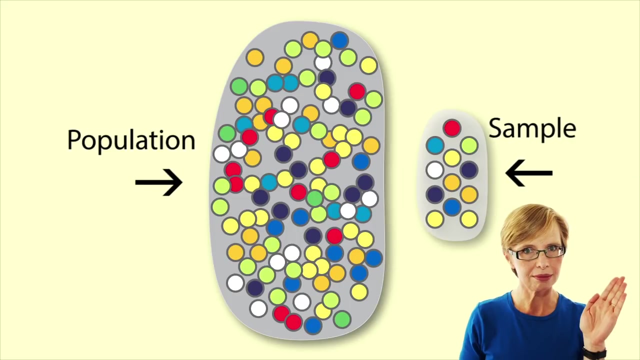 to the population from which it was drawn. A definition of inference is the process of drawing conclusions about population parameters based on a sample taken from the population. The sample is the data we collect from the population. Here are some examples of populations and samples. 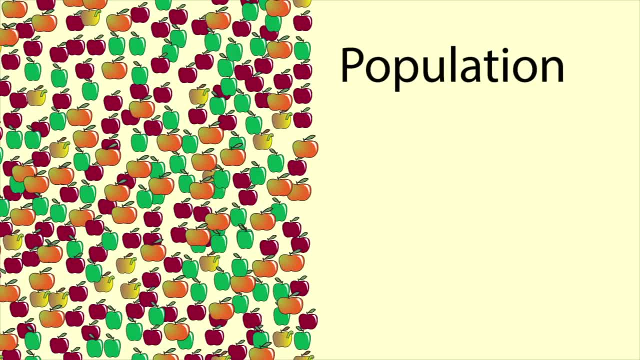 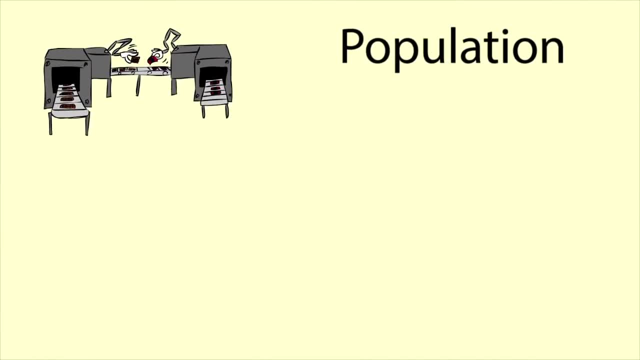 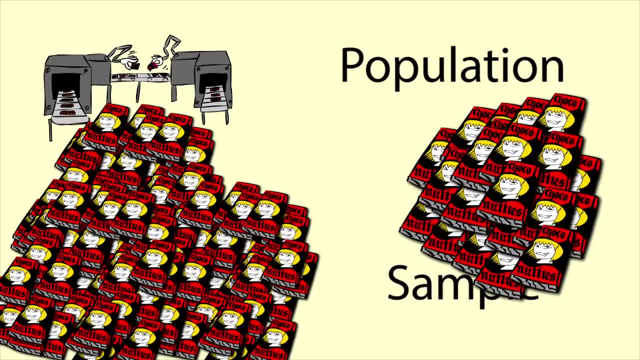 The population is all the apples in an orchard. A sample is 100 apples we pick from the orchard. The population is all the chocolate bars we produce on a machine. A sample is the 30 bars we choose to melt down and weigh the nuts from. 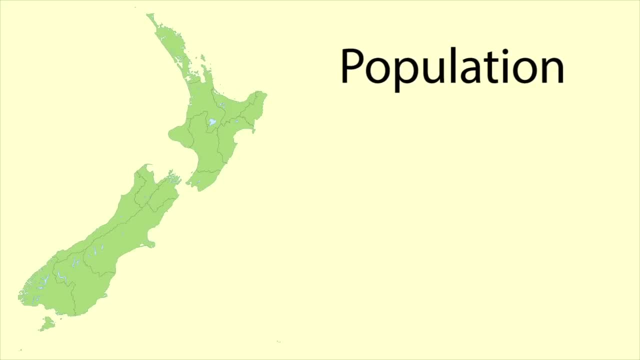 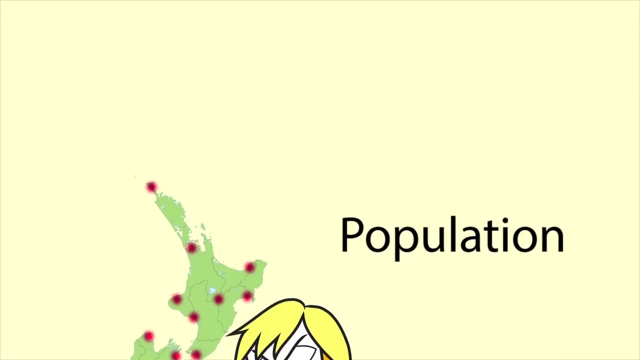 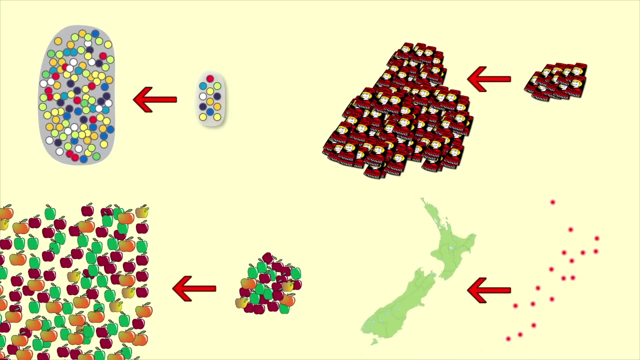 The population is all the voters. in New Zealand, A sample is 1000 people who are asked their opinion in an online survey. In each of these examples we can use the data from our sample to draw some conclusions about the objects or people in the population. For example, we want to know about the 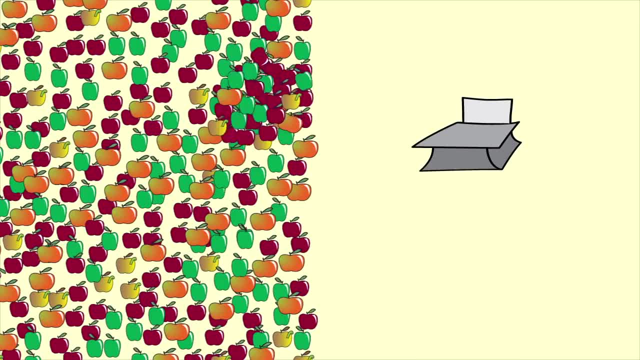 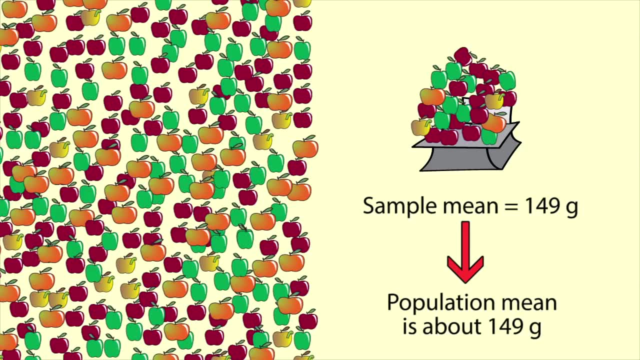 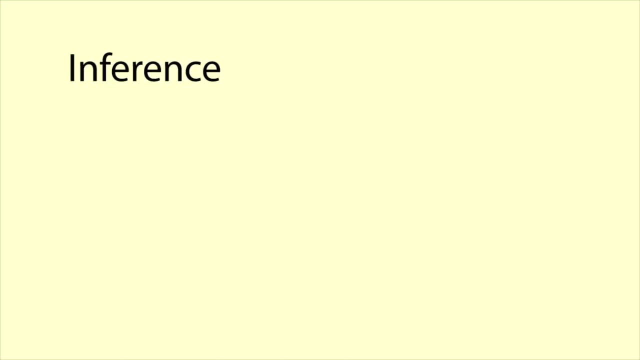 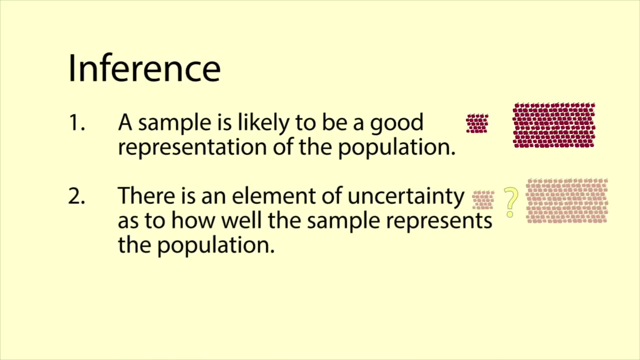 weights of the apples in the orchard. so we take a sample of apples and weigh them and use that information to draw conclusions about the weights of apples in the whole orchard. There are three main ideas underlying inference: A sample is likely to be a good representation of the population. There is an element of 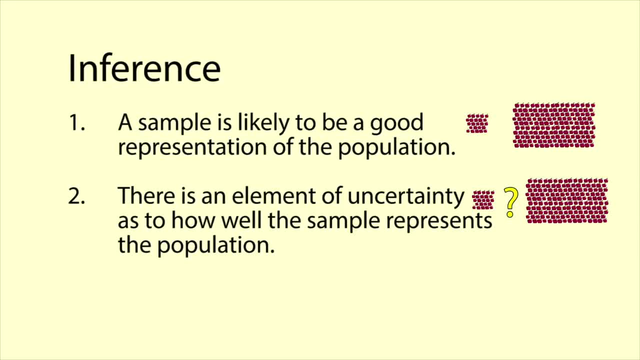 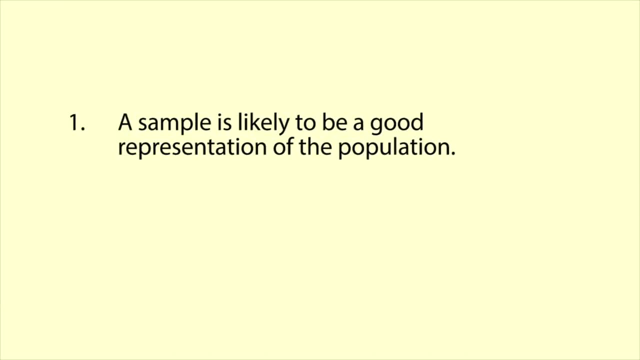 uncertainty as to how well the sample represents the population and the way the sample is taken matters First. it is reasonable to expect that a sample of objects from a population will represent the population. If our orchard has only red apples of a fairly consistent size, then we would expect the 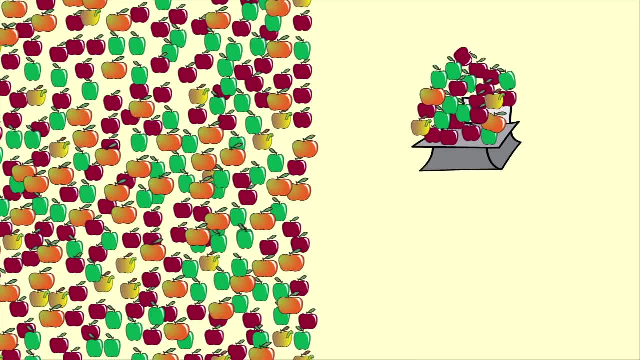 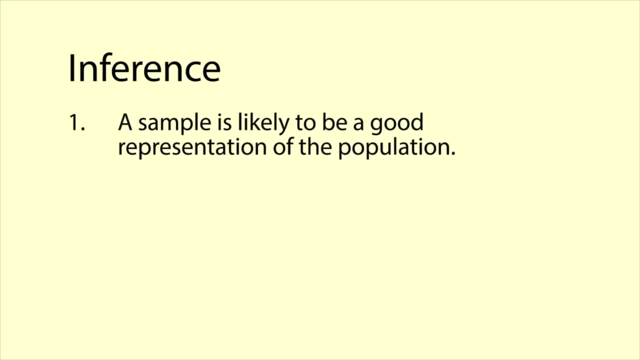 in the orchard. so we take a sample of apples and weigh them and use that information to draw conclusions about the weights of apples in the whole orchard. There are three main ideas underlying inference: A sample is likely to be a good representation of the population. 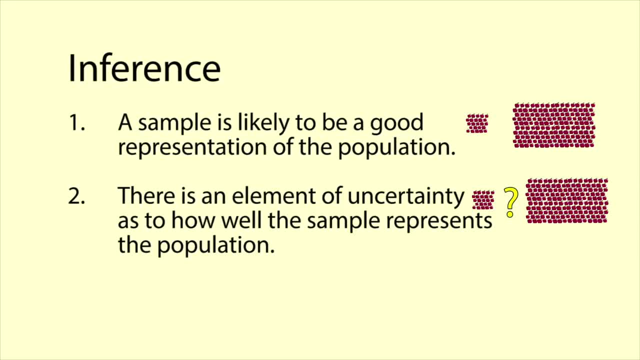 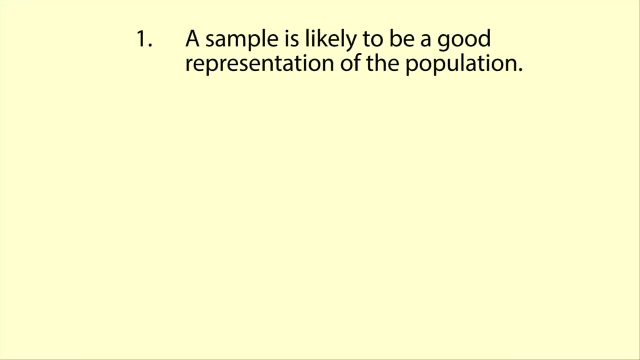 There is an element of uncertainty as to how well the sample represents the population, And the way the sample is taken matters. First, it is reasonable to expect that a sample of objects from a population will represent the population If our orchard has only red apples of a fairly consistent size. 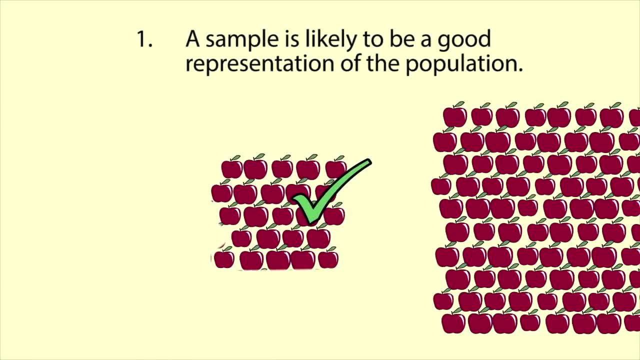 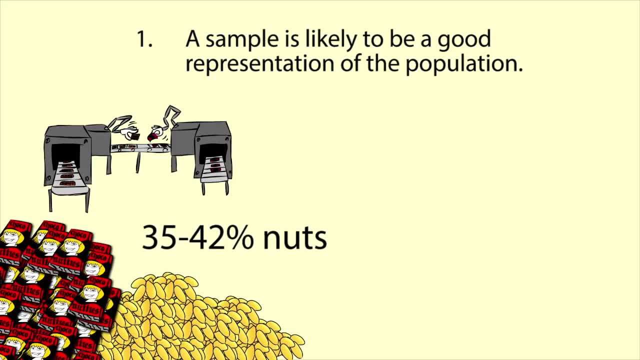 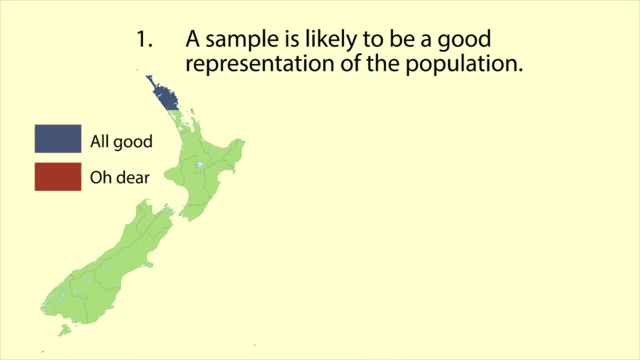 then we would expect the sample to contain red apples of a fairly consistent size. If our machine is producing chocolate bars with a percentage of nuts within a certain range, then we would expect the sample to also have nuts within that range. If 40% of the people in New Zealand believe that the economy is getting worse, 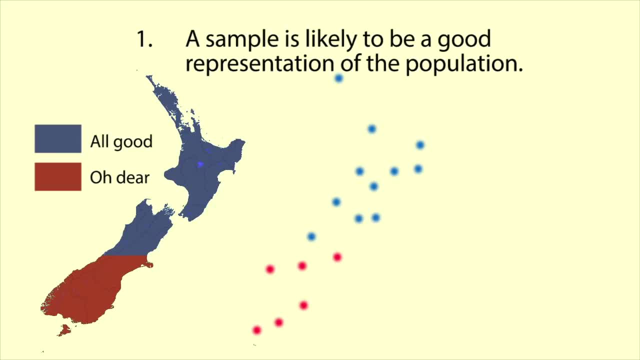 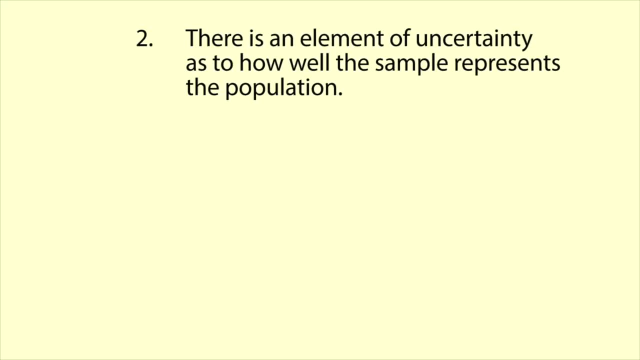 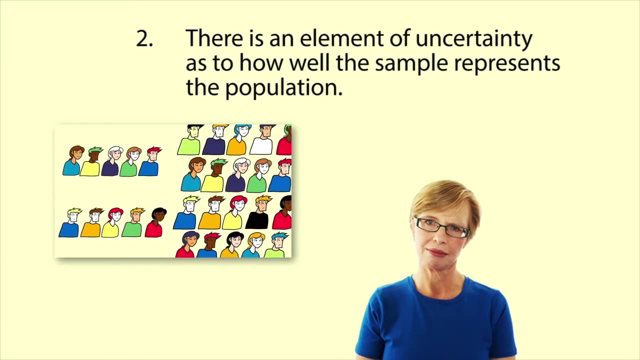 then about 40% of the sample will also believe that. Second, there is an element of uncertainty as to how well the sample represents the population. A sample will never be a perfect representation of the population. A sample will never be a perfect representation of the population from which it is drawn. 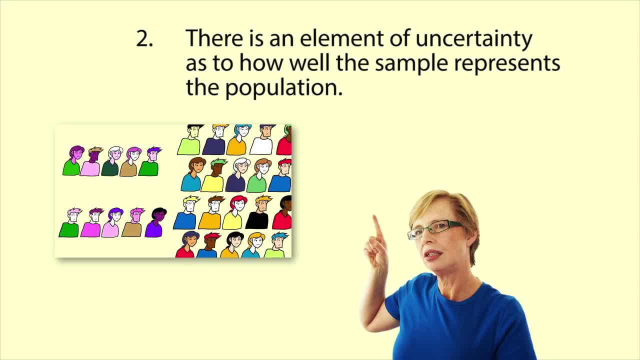 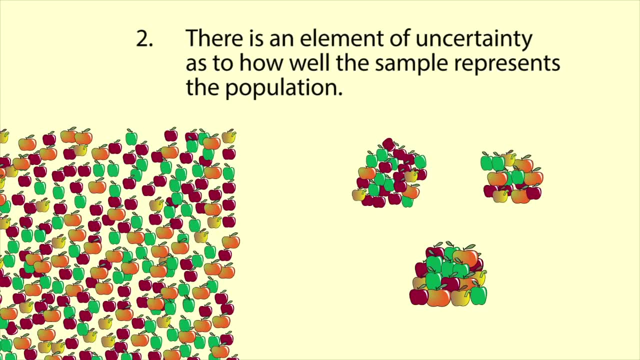 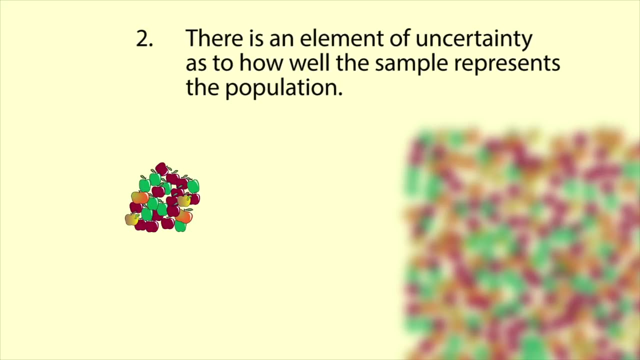 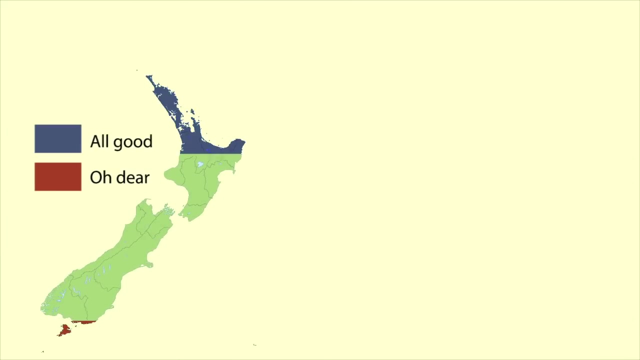 This is the reason for sampling error. We have a video about sampling error. Nor will all the samples drawn from the same population be the same, But through simulation and probability theory we can get an idea of what the population is likely to be like from the information the sample gives us. For example, let us assume that 40%. 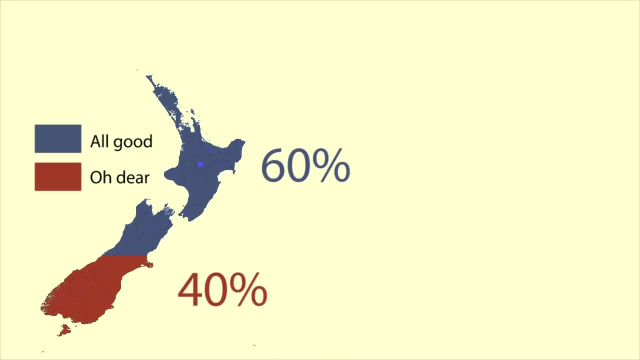 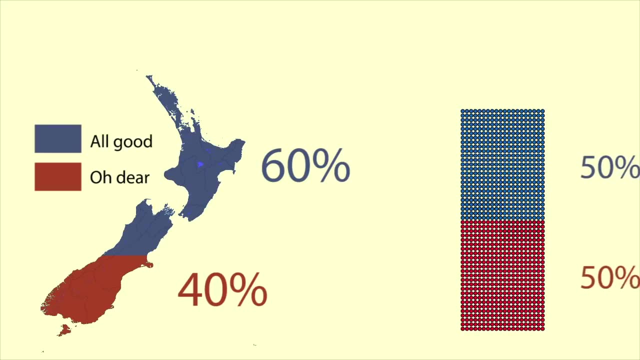 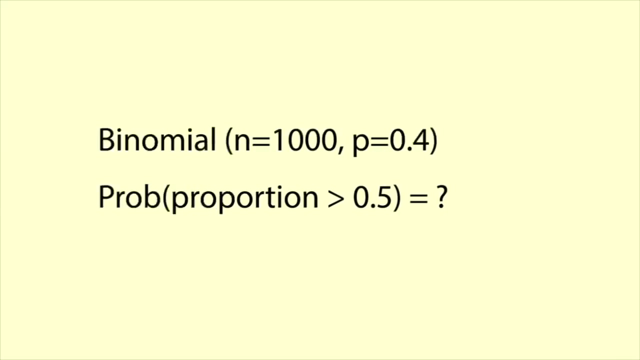 of the population of New Zealand think the economy is getting worse. If we took a sample of 1,000 people, how likely is it that 50% or more of them will say that they think the economy is getting worse? We can work this out using probability theory. 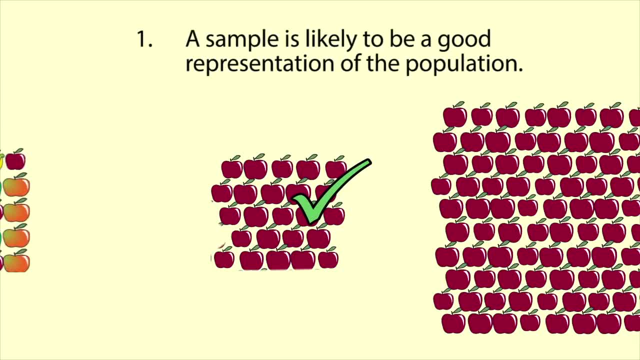 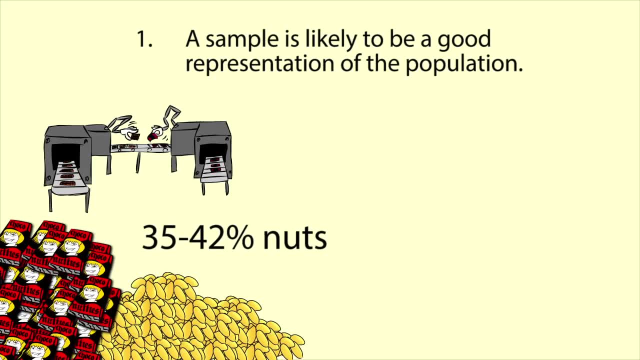 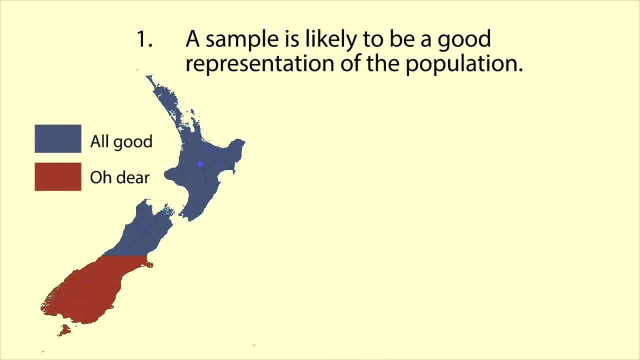 sample to contain red apples of a fairly consistent size. If our machine is producing chocolate bars with a percentage of nuts within a certain range, then we would expect the sample to also have nuts within that range. If 40 percent of the people in New Zealand believe that the economy is getting 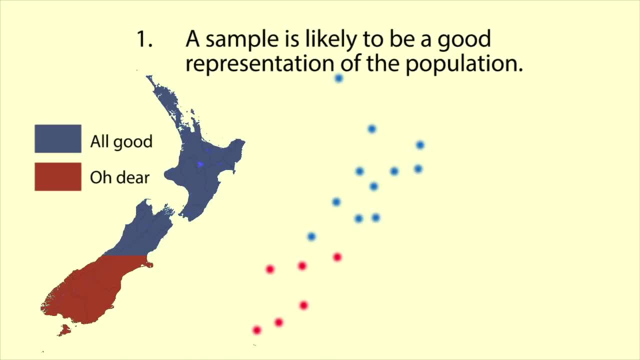 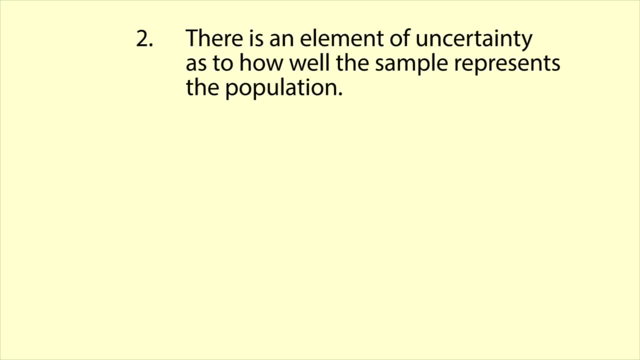 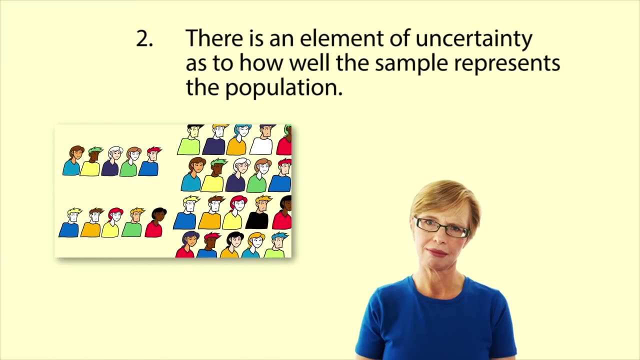 worse, then about 40 percent of the sample will also believe that. Second, there is an element of uncertainty as to how well the sample represents the population. A sample will never be a perfect representation of the population from which it is drawn. This is the reason for sampling error. We have a 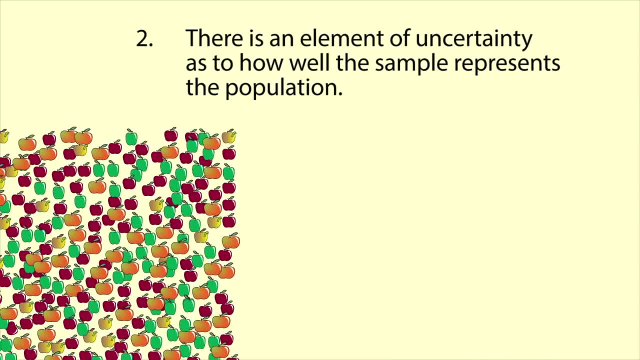 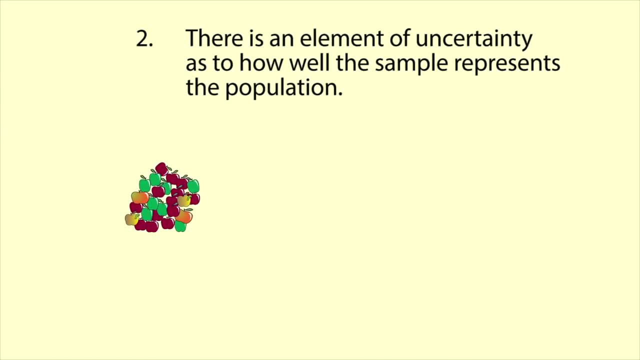 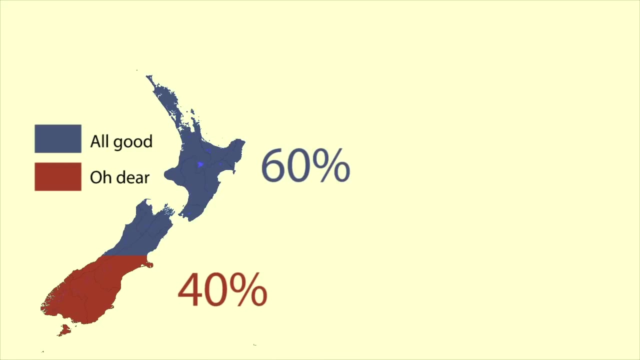 video about sampling error. Nor will all the samples drawn from the same population be the same, But through simulation and probability theory we can get an idea of what the population is. For example, let us assume that 40 percent of the population of New Zealand think the 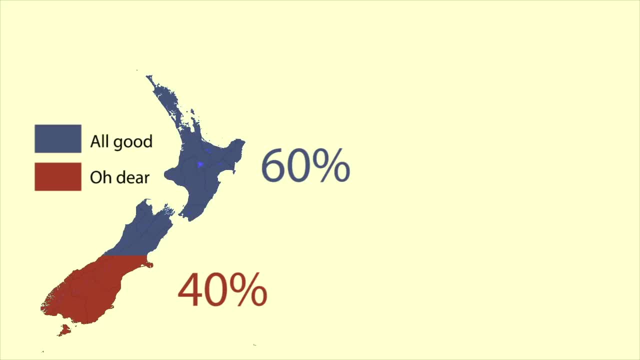 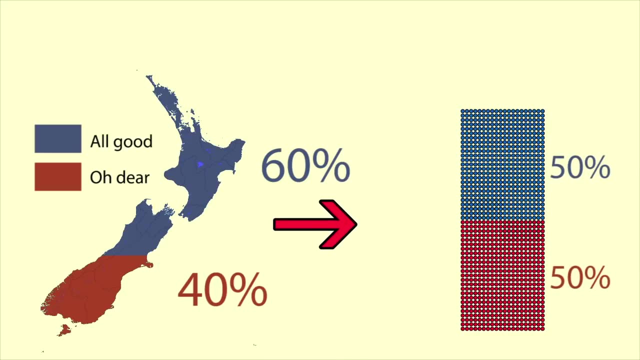 economy is getting worse. If we took a sample of 1,000 people, how likely is it that 50 percent or more of them will say that they think the economy is getting worse? We can work this out using probability theory or we can run a. 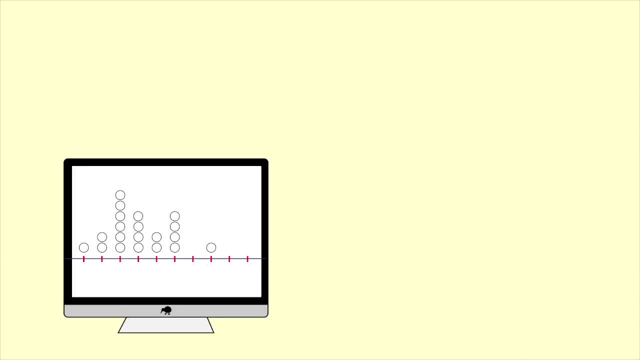 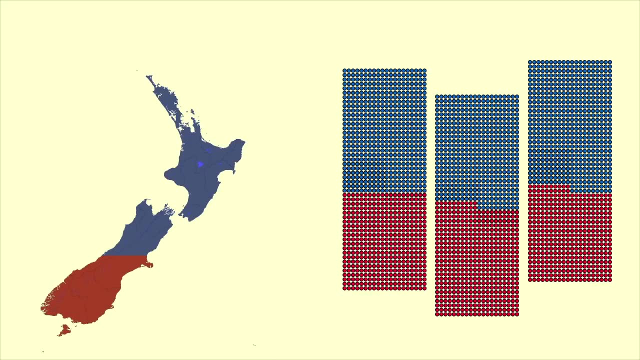 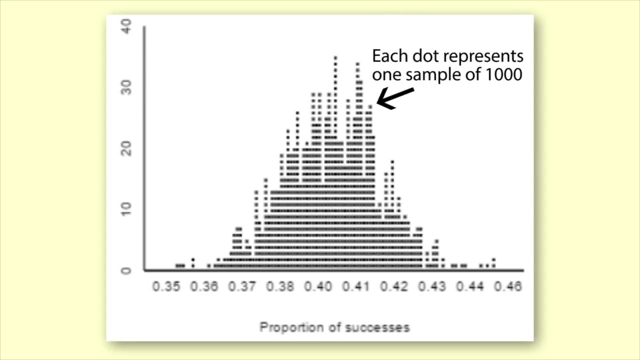 simulation on a computer to see what we would expect from a whole lot of samples of size 1,000, taken from a population with 40 percent thinking the economy is getting worse. This graph is the result of a simulation with a thousand samples of a thousand people, each drawn from a 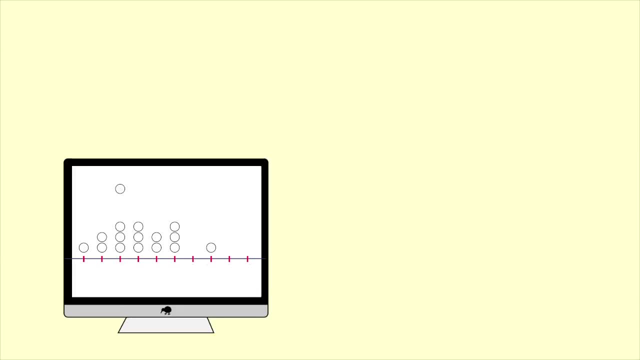 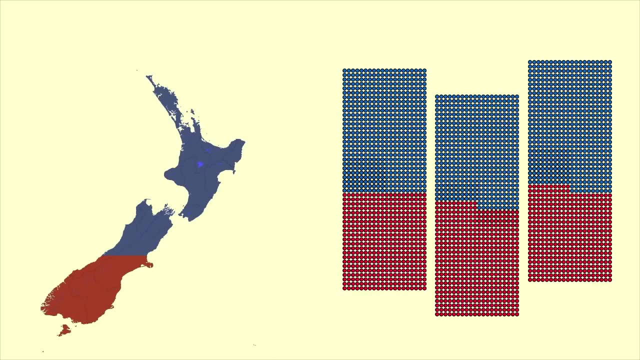 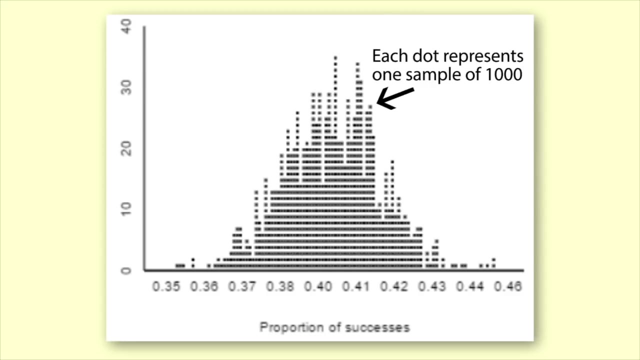 or we can run a simulation on a computer to see what we would expect from a whole lot of samples of size 1,000, taken from a population with 40% thinking the economy is getting worse. This graph is the result of a simulation with 1,000 samples of 1,000 people each. 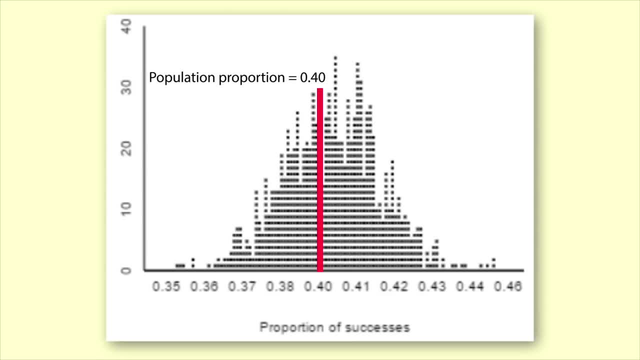 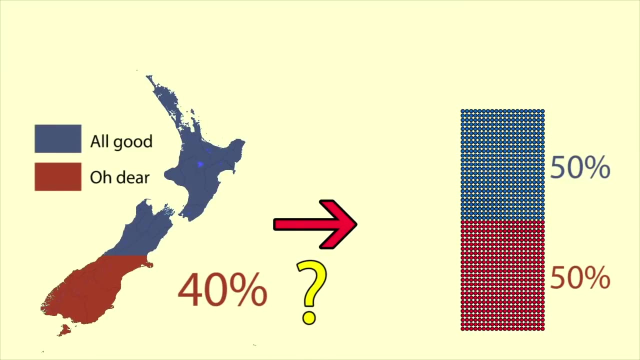 drawn from a population with a proportion of success of 0.4 or 40%. We define success as being that the person thinks the economy is getting worse. It turns out that if the true proportion in the population is 40%, the probability of getting a sample with 50% or more people saying that they think the economy is getting worse is 50%. 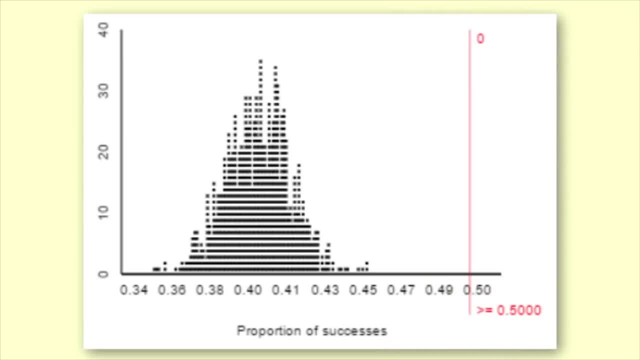 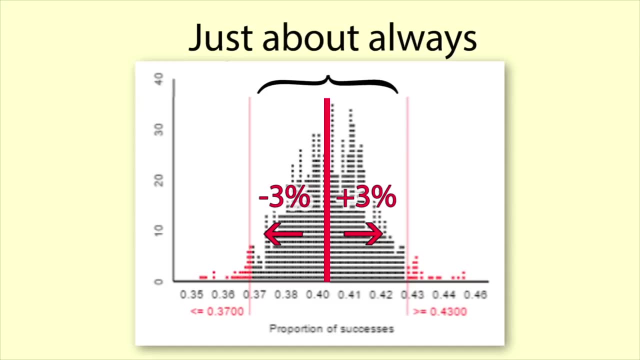 If the result is that the economy is getting worse, it is 0. It won't happen. Just about always. the sample proportion will be within about 3% of the population proportion when we use a sample size of 1,000.. That 3% is called the margin of error. 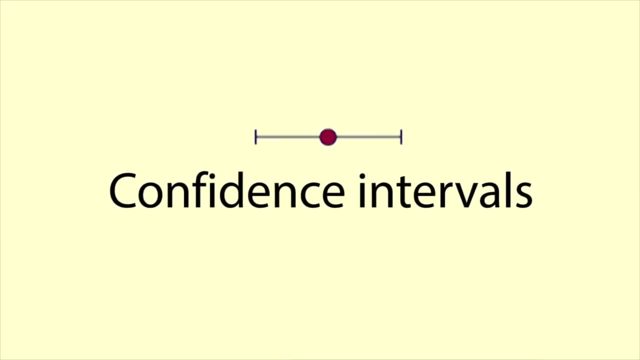 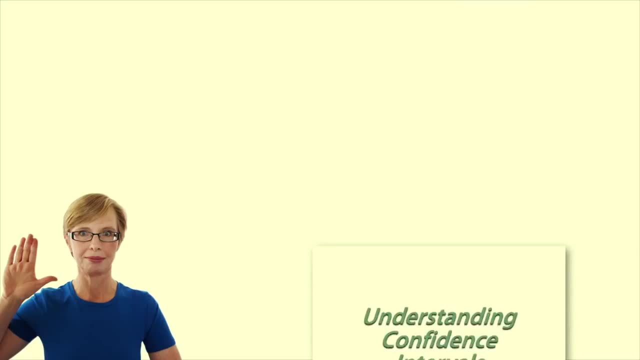 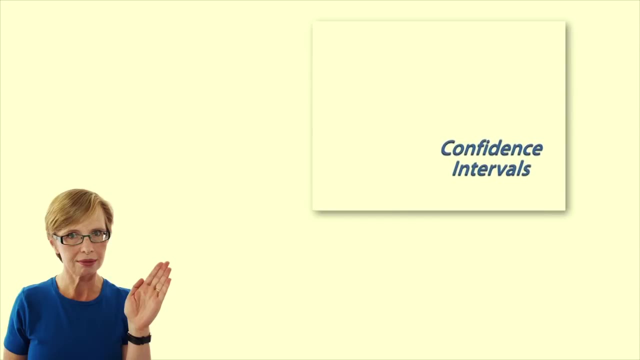 It can be used to create confidence intervals. Confidence intervals give a range within which we think the population parameter is likely to be. You can see more about confidence intervals in our video Understanding Confidence Intervals In inferential statistics. we can also test hypotheses. 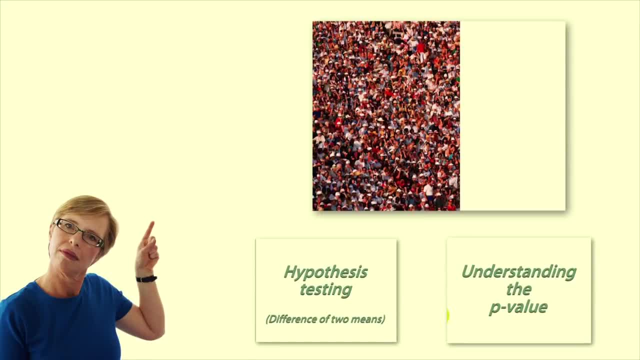 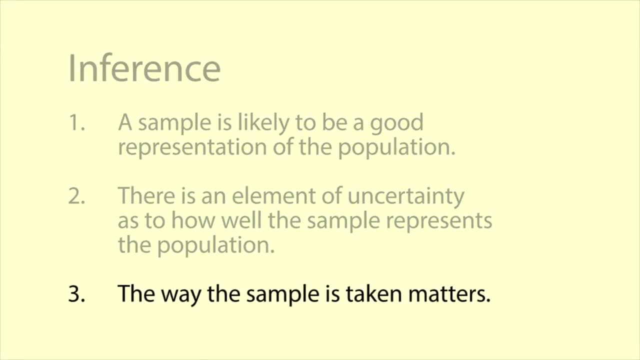 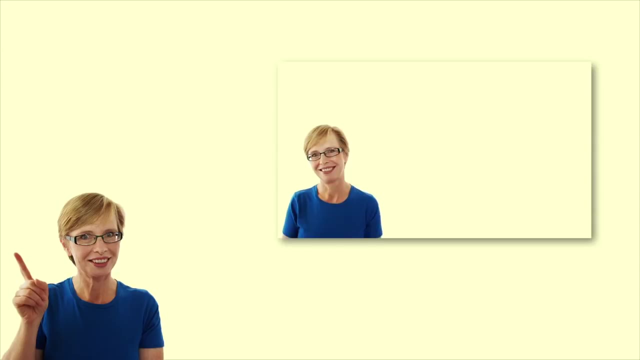 Our videos Understanding the P-value and Hypothesis Testing explain these. The third principle is the way the sample is taken matters. This principle relates to non-sampling error, which we also have a video about. The sample must be represented. 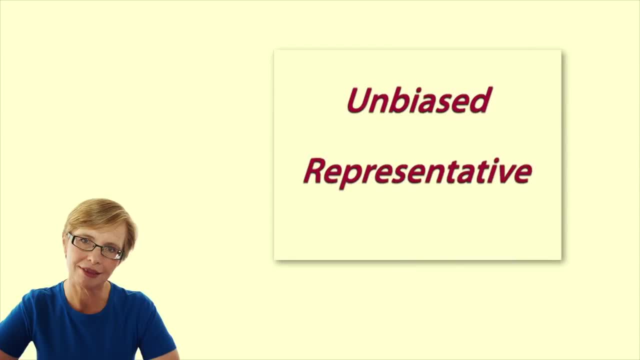 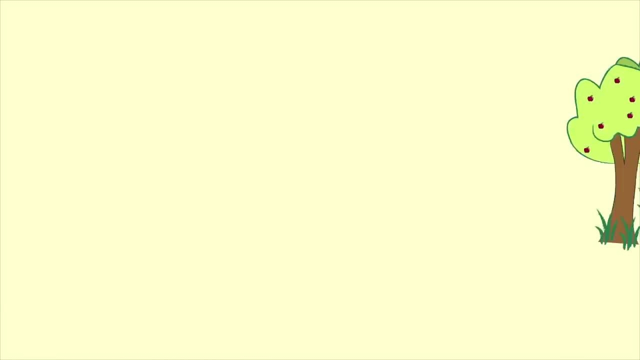 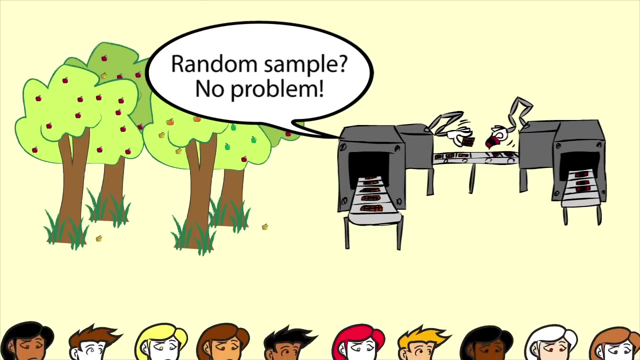 The sample must be representative of the population, And this happens best when each person or thing in the population has an equal chance of being selected in the sample. In natural or manufacturing processes, we may be able to take random samples reasonably easily. However, when our population consists of people, this can be more difficult and costly. 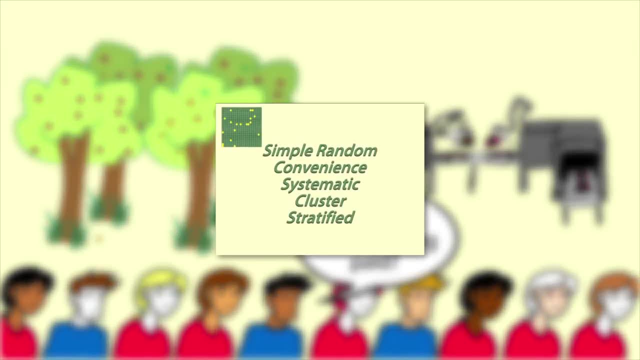 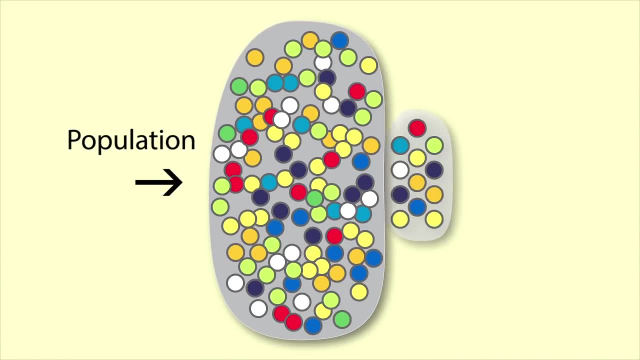 so we do the best we can. We explain this further in our video on sampling methods. The sample method is an example of sampling methods. This video has been about sample to population inference. We are interested in what the sample tells us about the population. 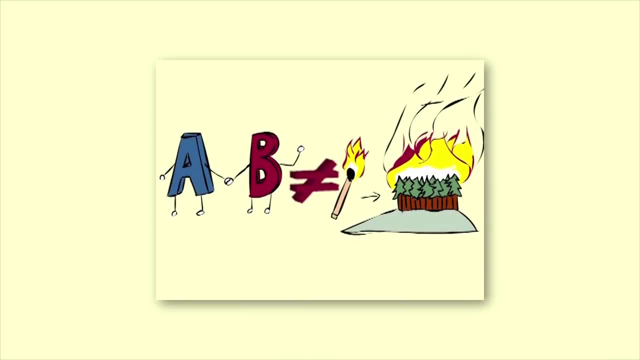 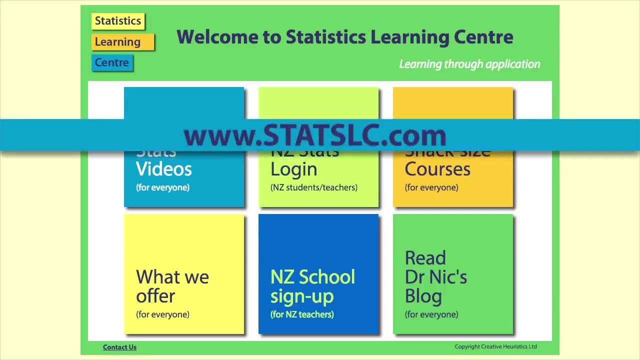 It is not about causation, which is covered in other videos. This video was brought to you by Statistics Learning Centre. Visit our website for more resources to help you learn. 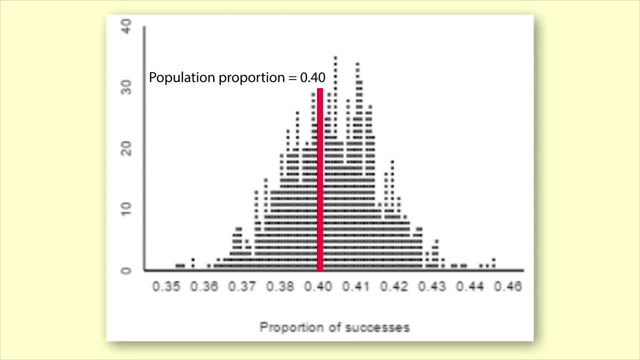 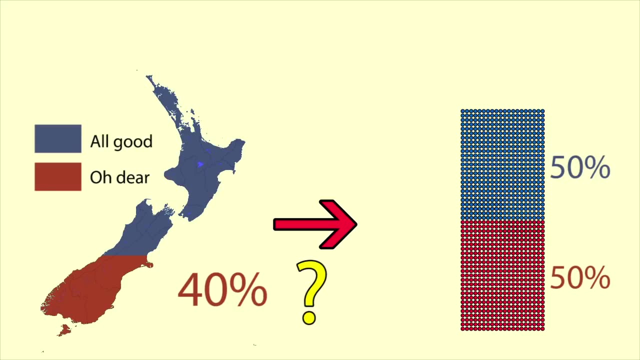 population with a proportion of success of 0.4 or 40 percent. We define success as being that the person thinks the economy is getting worse. It turns out that if the true proportion in a population is 40 percent, the probability of getting 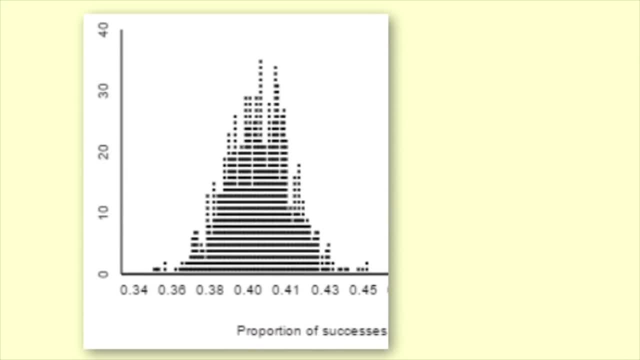 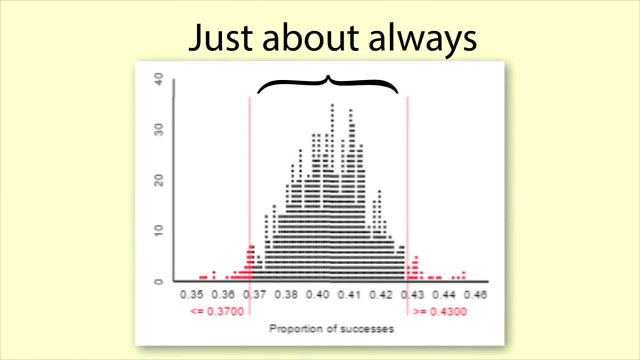 a sample with 50 percent or more people saying that they think the economy is getting worse is… zero. It won't happen, Just about always. the sample proportion will be within about 3 percent of the population proportion when we use a sample size of 1,000.. That 3.